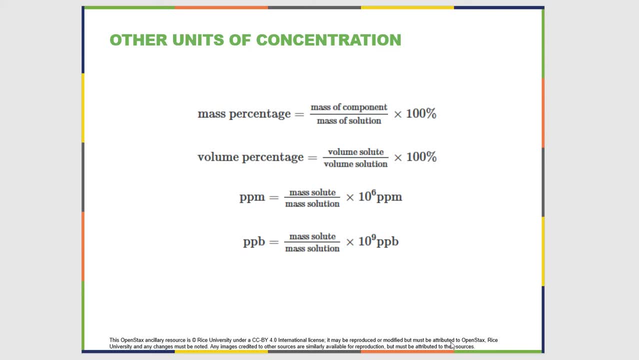 In the previous section. in the previous section we talked about the unit of concentration of molarity. In this section we want to look at it. some other units of concentration, and I'm not going to say that these units of concentration are useless, because they're certainly not. They're used all the time in 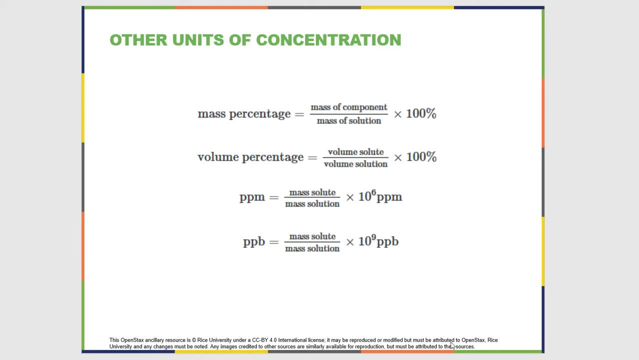 professional ways, but they're not used very often in this course. In fact, the only other unit of concentration that's used extensively in this course is molality, which we'll talk about for later on. But here we're looking at some other units of concentrations like mass percentages and volume percentages. These 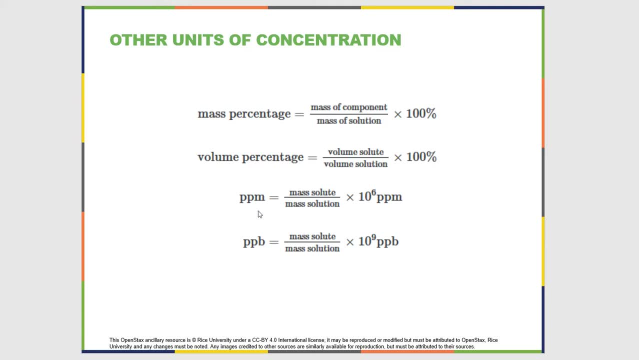 are very common in the healthcare industry: Parts per million and parts per billion. these are very common in environmental science type of applications. So I do want to give you an idea that they exist and give you one example of mass percent which we actually use in the lab course here. 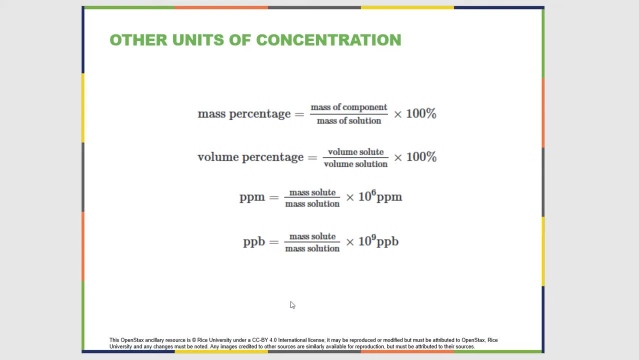 not so much in the lecture but in the lab course, And so you just have one example of you know how this stuff can be useful. So mass percentage or volume percentage is the mass of the component, the part divided. 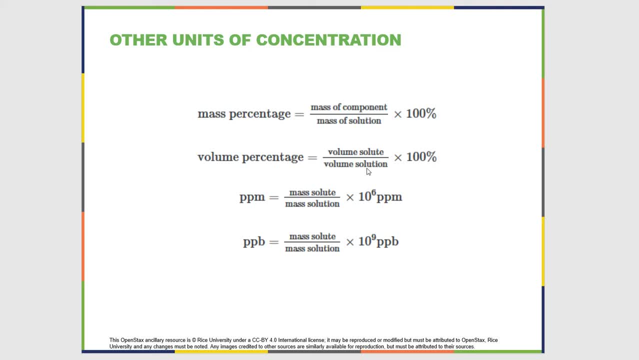 by the mass of the solution, the whole, or the volume of the solute of the volume of the solution, which is the part, again, but divided by the whole. So, and of course they're times 100, because they're percentages. So again these are used. 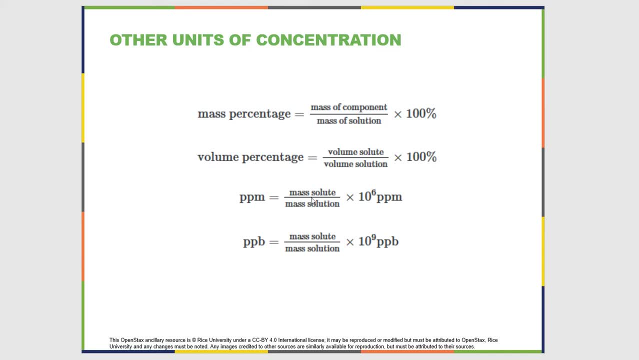 often in the healthcare industry. Parts per million is mass of solute over mass of solution, the part divided by the whole times 10 to the 6.. 10 to the 6, here being a million. Parts per billion is the mass of the solute divided by the mass. 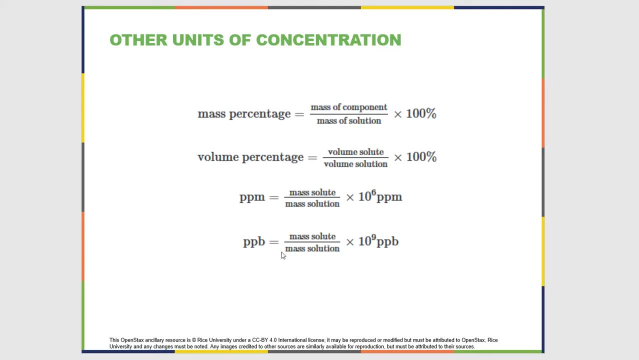 of the solution times 1 billion. So if the the solution is water, this is usually considered as a milligram per kilogram and in fact it doesn't have to be water for that to be the case. So this is a milligram per kilogram. so if 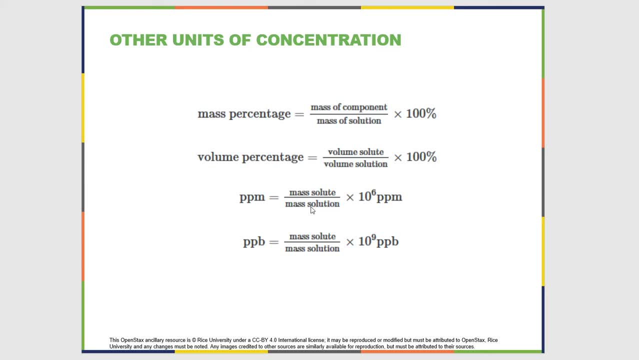 something is one part per million in water, that means there's one milligram of it in a kilogram of the water sample or the solution. If it's a part per billion, that's a microgram per kilogram. so that's again if you have a kilogram. 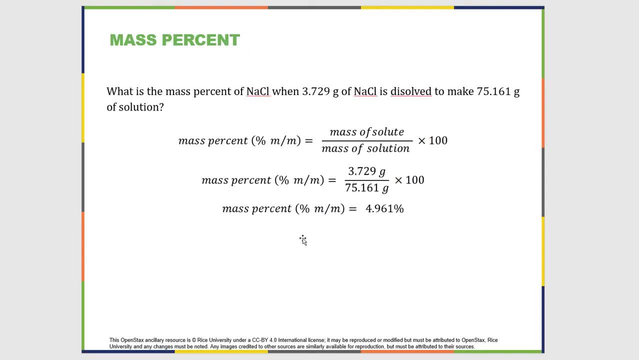 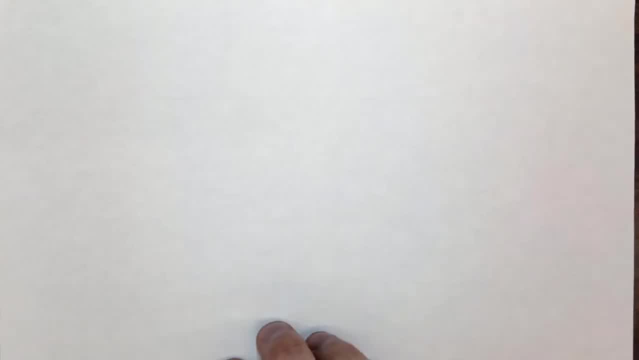 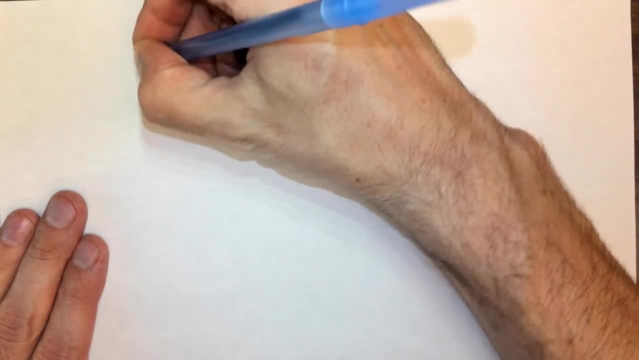 of water, that's one microgram per kilogram. Here we're gonna look at a mass percent question, but like usual, we're gonna do it on a piece of paper as opposed to doing it on the on the slide. So it's it. wants to know the mass percent?